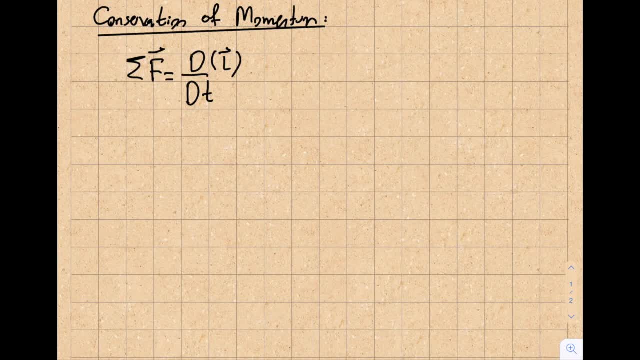 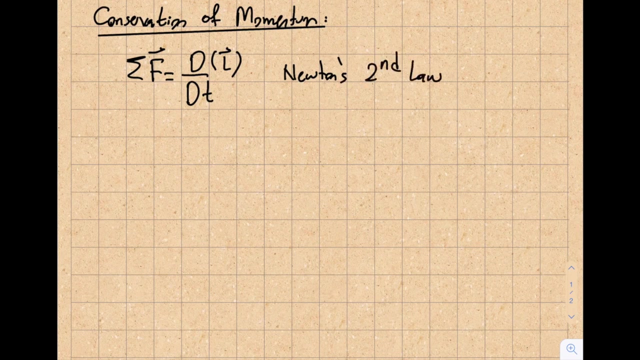 so they will have components in the directions that you're interested in, such as x, y, z or r, theta z in the polar coordinates. Okay, so basically this is the Newton's second law. Now I'm going to actually insert what's. 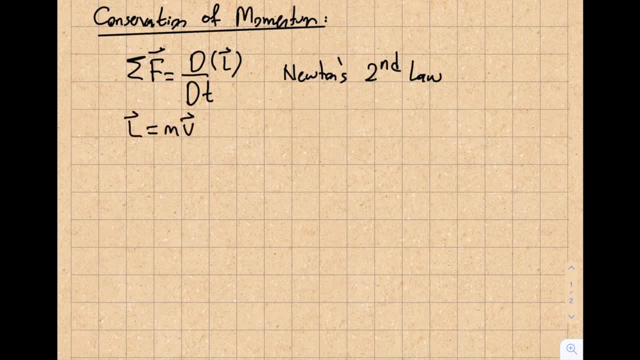 linear momentum is- and you may remember from your physics courses that linear momentum is equal to mass times the velocity. Okay, so this formula then becomes summation of the forces, becomes d, dt. Remember, this is a material derivative, because this is applied to a particular point in the flow. Okay, and v, All right. next is I'm going to remind: 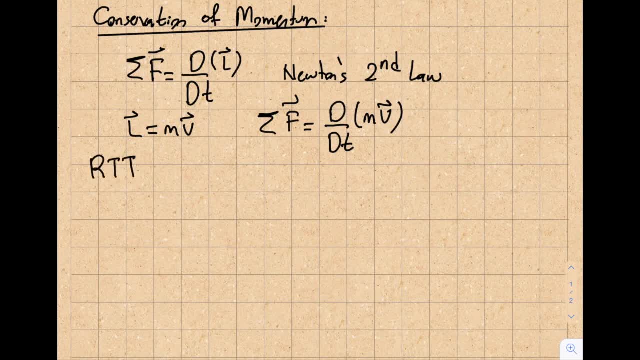 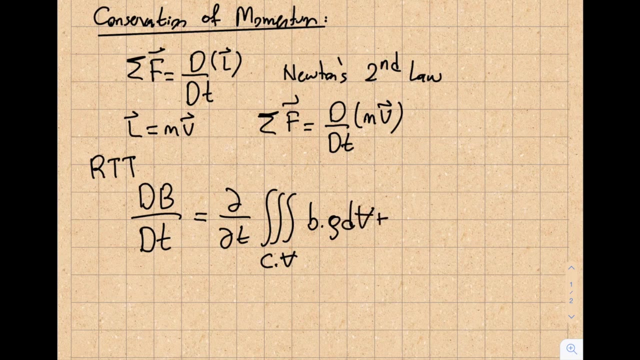 you the Reynolds transport theorem and see whether we can play with that. Okay so db dt v was just a placeholder del del t of triple integral over the control volume v, lowercase b v. volume plus control surface v, rho velocity, dotted with n, da Right, this was. 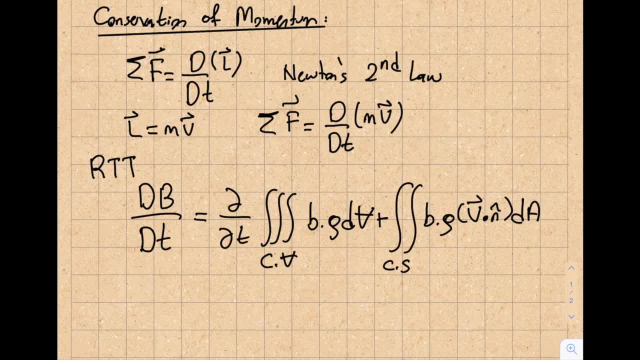 my Reynolds transport theorem and I can apply this to consider ratio of mass momentum, energy vector and potential velocity, and I will show you this again in the future. What I want to accomplish today is I'm going to be strategic and insert this capital. b is equal to this. 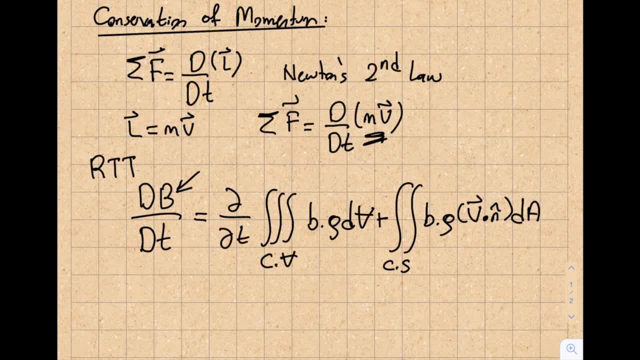 mv. Okay, because if you take a look at it, if I simply go out and insert this right over here, what will happen is, on the left hand side of the equation, is going to get- I'm going to get- d? dt of m times v, which is the linear momentum, And this n? mt power is equal. to V, n i, d t of r y. This is the linear momentum, and this n mt of r y is equal to v, and this is theós vs v. This is the quality of the equation. Okay, so what we do here is we take 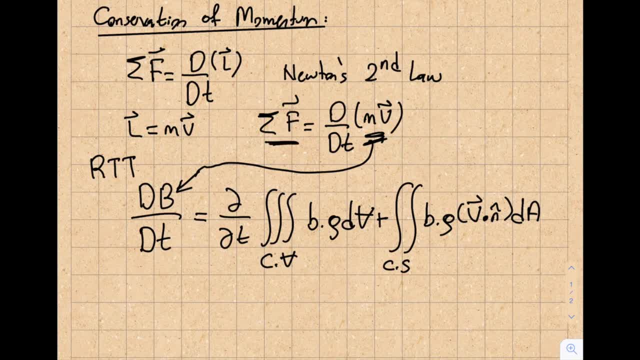 this, and we define the self-interference term and we call it the linear momentum of this value, and gonna go and say that this is equal to sum of the forces that will be giving me something useful for me to work with. okay, so let me repeat what I said, this: 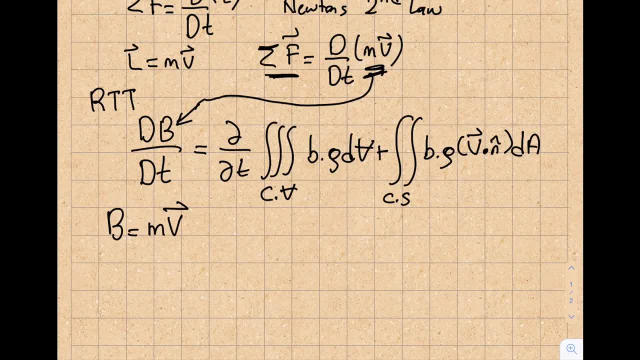 capital B is equal to M times velocity vector and if you remember from our earlier discussions, the ratio between the capital B and lowercase B is per unit mass. okay, and I'm gonna insert here M velocity vector and from here I'll get the lowercase B as velocity vector. right, you can see I'm still cancel out, okay. 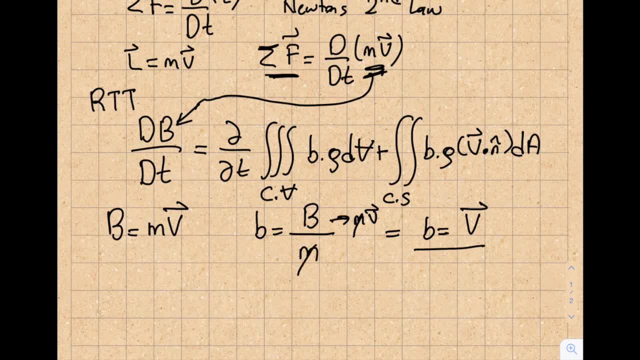 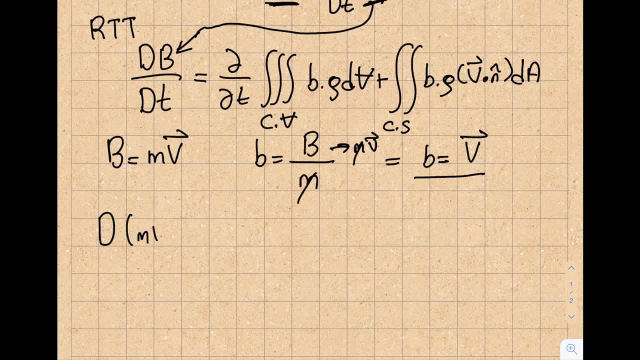 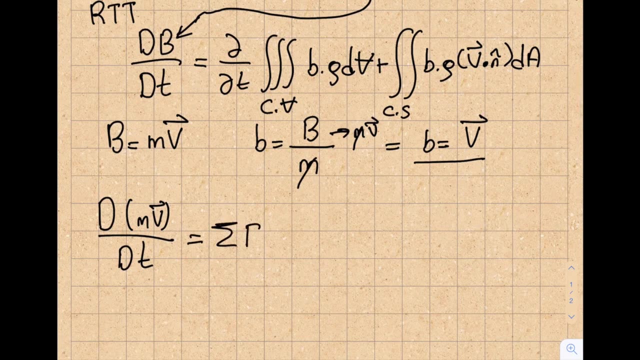 all right, so now I seem to know everything that I need to proceed. okay, so I'm gonna say that D, MV, DT, which is the linear momentum. I'm gonna use Newton's second law and say that this is going to be equal to the summation of. 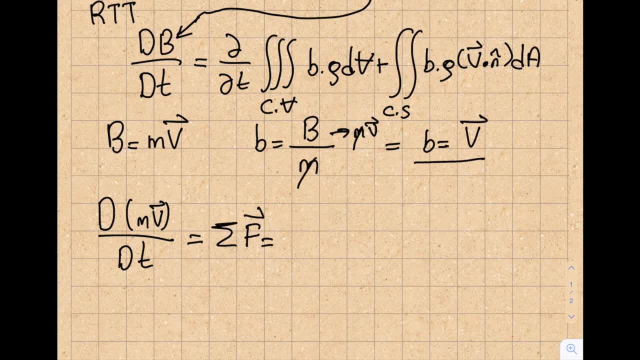 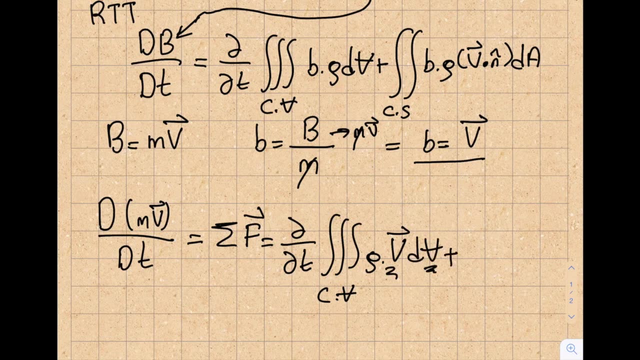 the forces now and then I'm gonna write the right hand hand side of the equations what's going to be done. let me no pass in the sum current- sorry, not the children's- leading from the equation now, plantillion, ill dealt E and again, triple control volume for 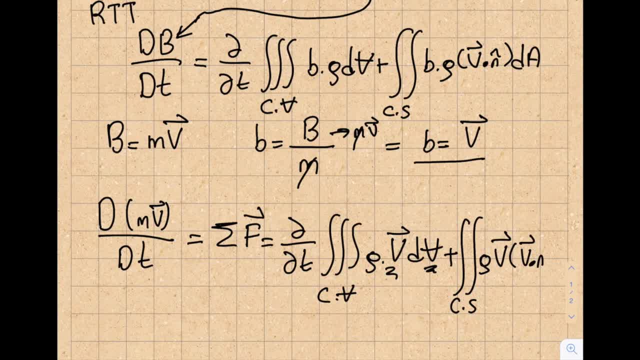 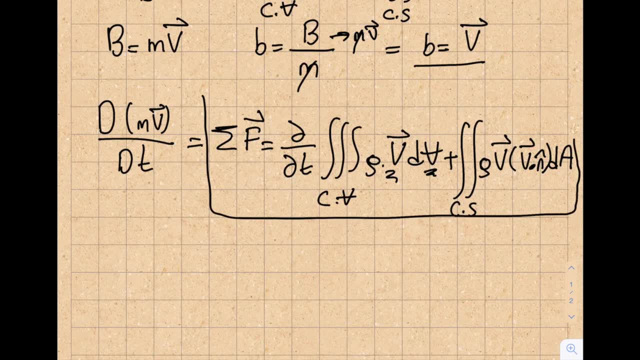 velocity vector viewpoint. be careful about these symbols. they look close to each other right and control surface raw velocity vector velocity least momentum. what i would like you to note that this is a vector equation, as i mentioned before and for components in the x direction, y direction and z directions. so now i want to go ahead and 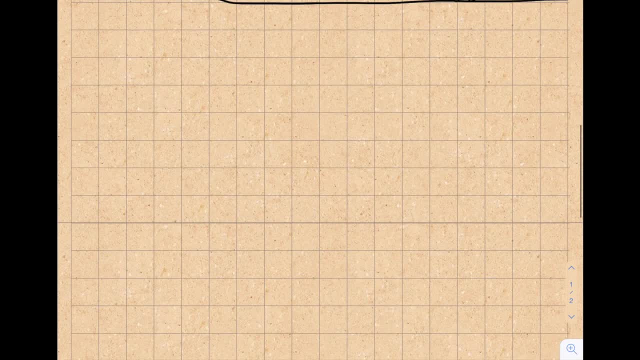 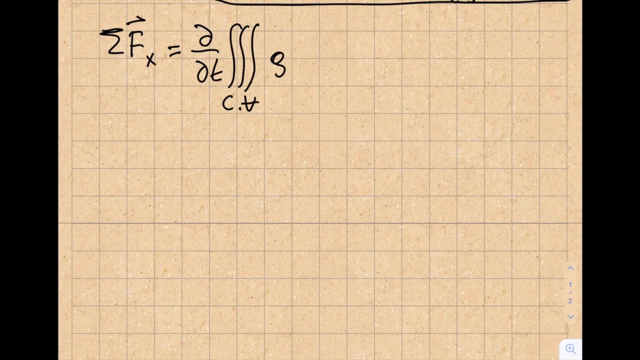 write these three equations if i'm using the cartesian coordinates. okay for your nodes for completeness purposes. so the summation of the forces in the x direction will be equal to del, del t, triple integral over the control volume, rho. v x d volume plus over the control surface: rho. 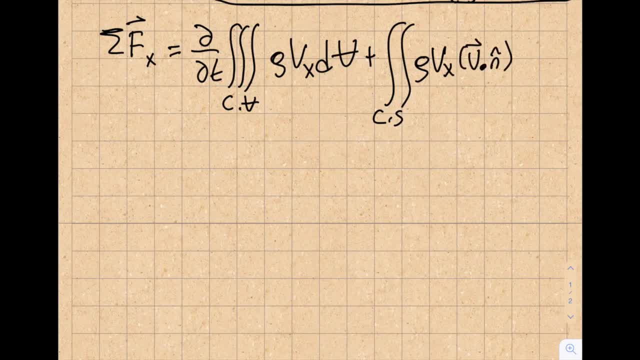 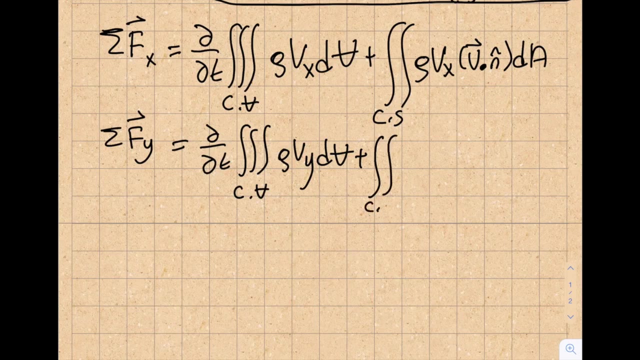 v x v, dotted with n d a. okay, you can have the similar equation in the y direction as well. so you'll get del del t of the control volume, rho v y d. volume plus over the control surface, rho v y d, dotted with n d a. and the third one will be summation of the forces in the z direction. 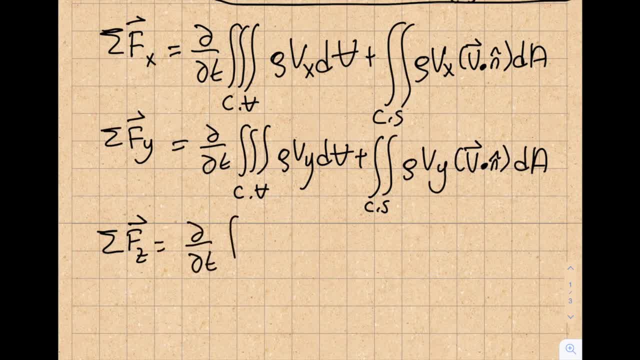 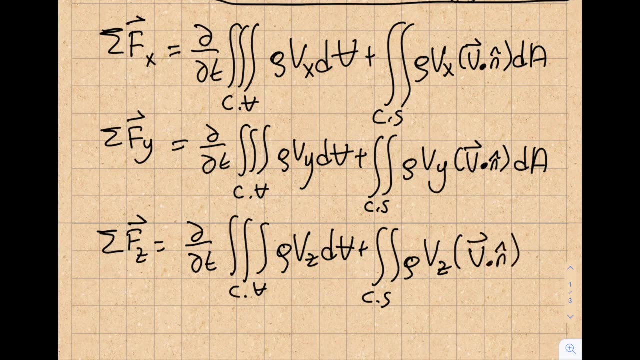 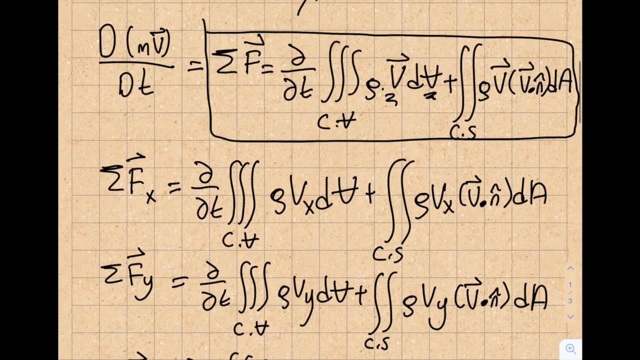 will be equal to del del t. one, two, three: control volume: rho v z d. volume plus over the control surface: rho v z v, dotted with n d a. okay, okay, now i have the three components that i need if i go up here, as i mentioned this. 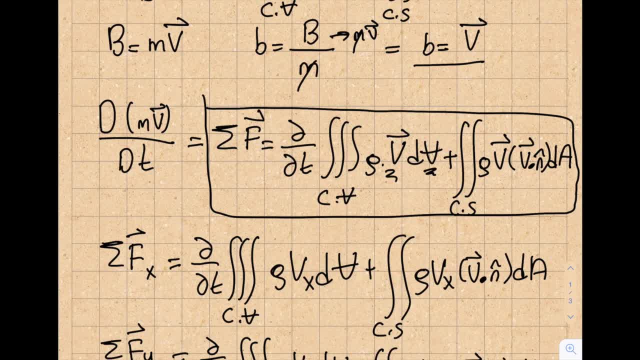 is a vector equation. when we look at the conservation of mass, we have seen that that is a scalar equation and typically what happens is that is the left hand side plus zero. okay is equal to: let's say the first term is plus five, the second term has to be minus five. 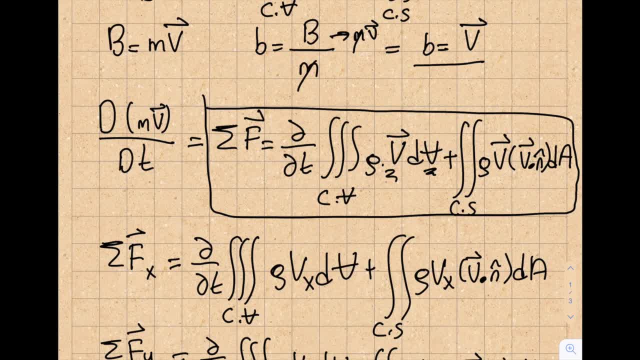 as simple as that, okay, um, in here it's a bit more complicated. okay, the left hand side is the summation of the forces. so, if you think about it, this is still the newton second law. okay, so this is equal. this is the flutes. equivalence of f is equal to m, a right. 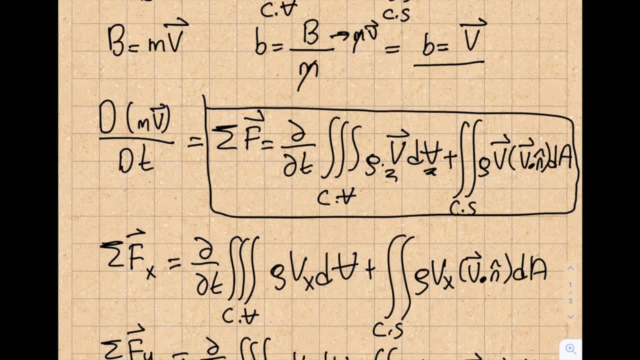 hand side is m a actually, if you think about it. okay, let's say that this is vector one, this is vector two, this is vector three. what happens is, let's say, the vector two is like this: okay, now let's say that vector three is this right, and then this is what it means. 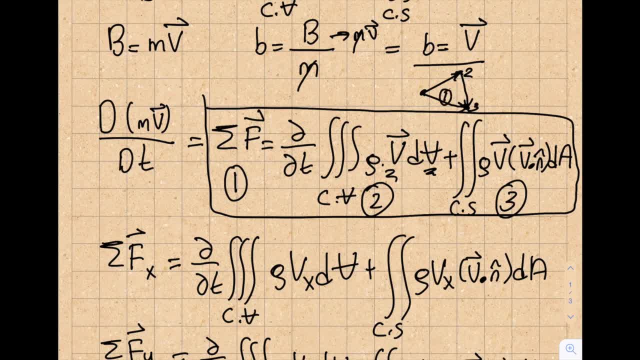 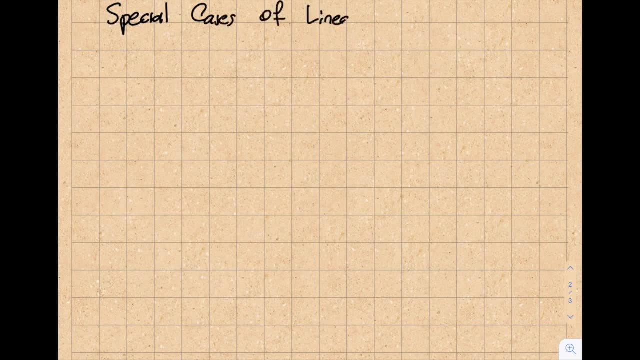 this one, or the summation of the forces, will be the summation of the vector two plus the summation of the vector three. okay, so this is quite different than the conservation of mass. i would like you to realize that, okay. okay, let's talk about the special cases of linear momentum. 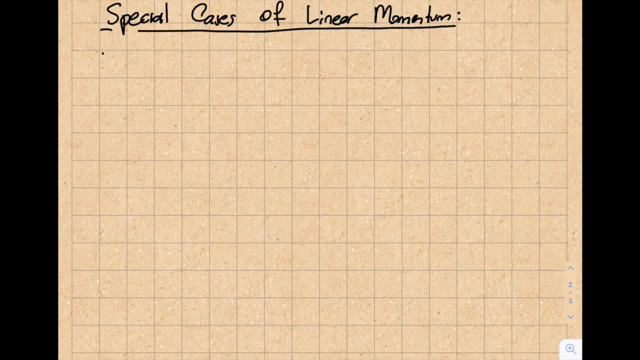 the first thing i want to highlight here is the first assumption or special case that we have evaluated when we're doing the conservation of mass was the steady flow, and i will do the same. okay, what did steady flow mean? as a another recommendation, did it mean that the velocity 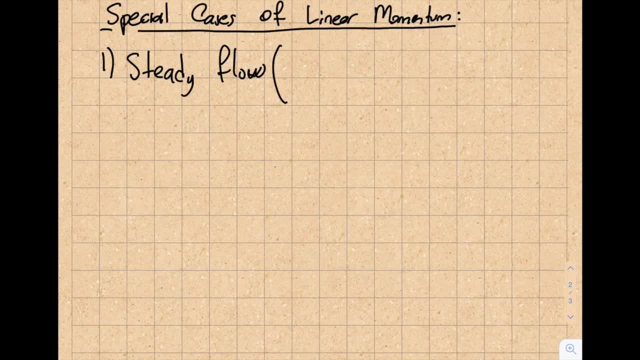 is constant throughout the flow. no, it doesn't, okay, and i gave the example. i was doing an experiment in my lab and i take a break, i go to the lunch. i came back from the lunch and nothing has changed, okay, in terms of the flutes, flow characteristics wise and properties wise. so that means that the 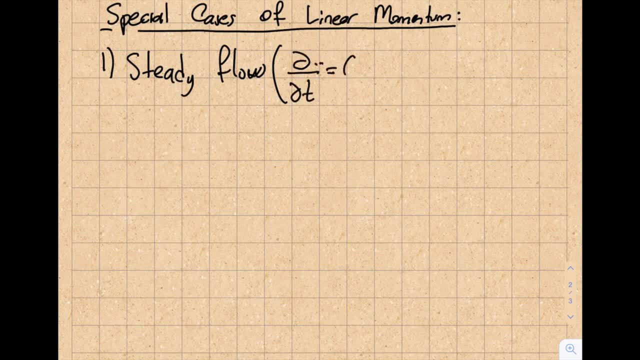 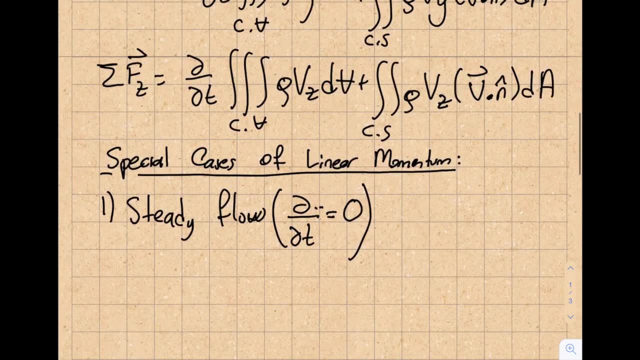 rate of change of things over time will be zero. okay. steady means that okay. and if I go up in here, if I look west, I look at the Z equation, you will see that the first term is looking at how does this triple integral changes over time for a? 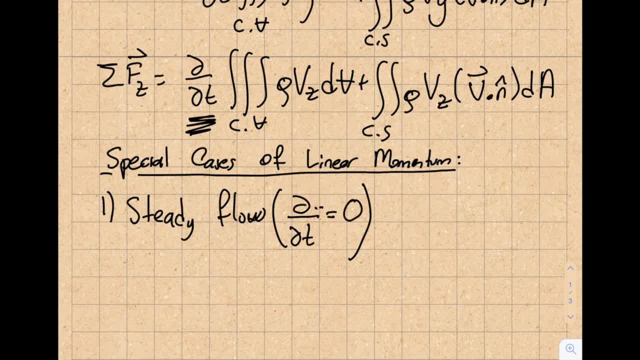 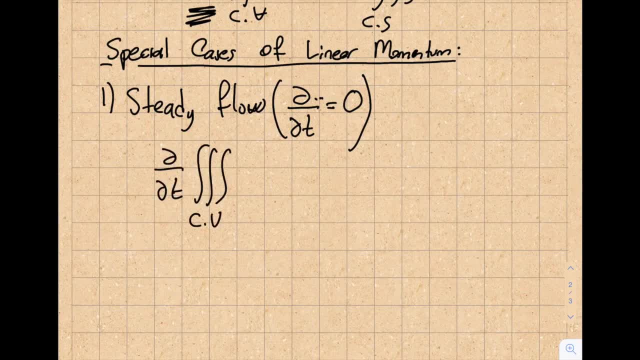 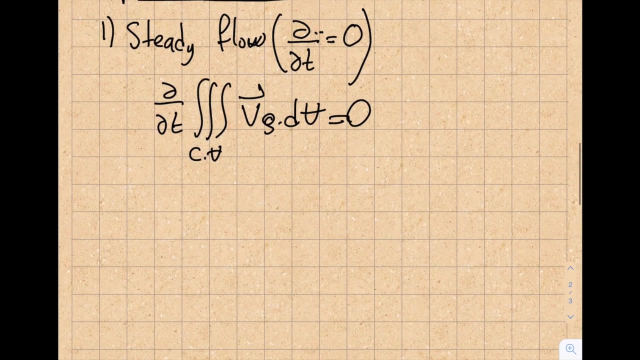 steady case, the answer would be: it doesn't change. okay, because del, of del T, of this triple integral over the control volume velocity vector, times Rho, times D, volume will be equal to zero. I'll talk about more this equation. okay, so you can see that I numbered it at number two vector turns out to be zero. 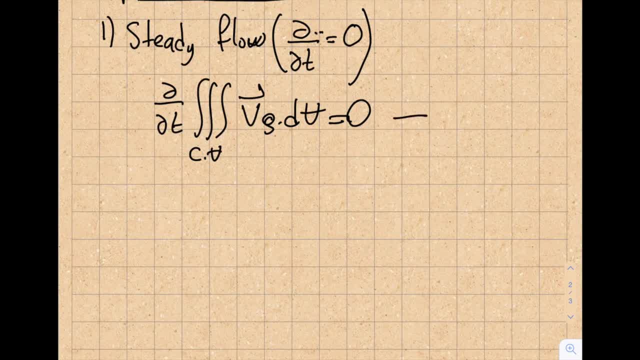 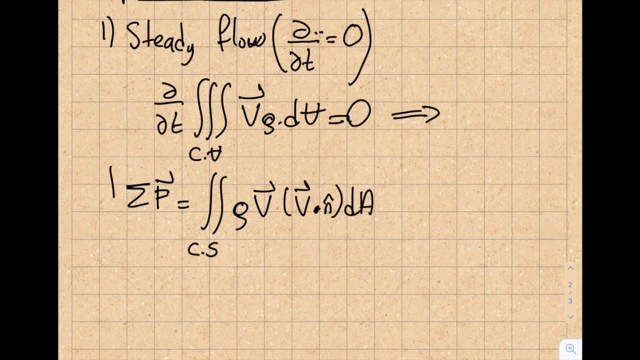 okay, and what it basically means. then my summation of the forces will be just this last term, so it will be over the control surface: Rho velocity, vector velocity, that and da. so this will be the equation that I obtain after I go through this process. okay, and I gave the example of vector 1, vector 3, if I use. 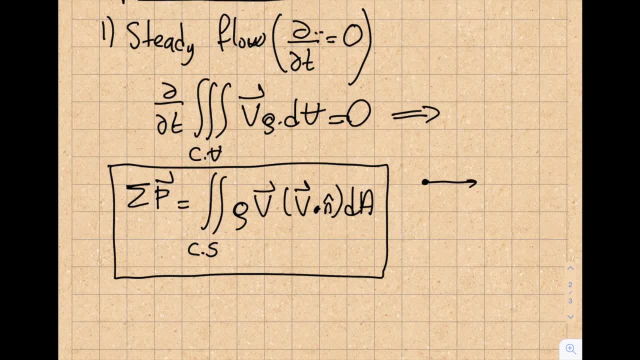 the same analogy. so what it says is: vector 3 and vector 1 is identical. so if 1 is 3, 1 is 1 because 2 is 0, right? so the vector 1 and vector 3 are the same. that's what it means. so when I was doing the constant ratio of mass, you may 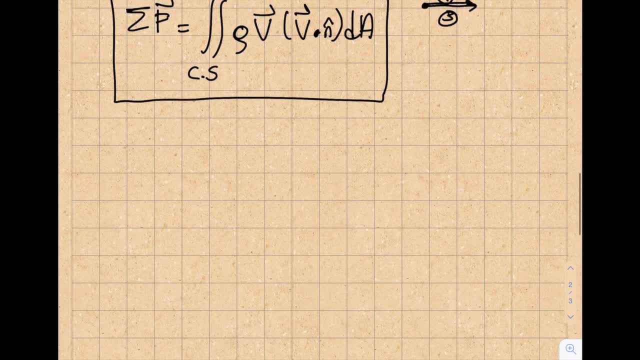 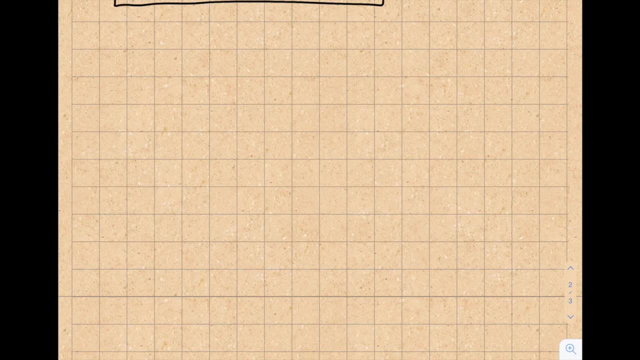 remember that I did steady plus incompressible flow right, so I don't really need to do it in here. because in that case there was a density was able to take out of the integrals. left hand side was 0, so I divided everything by the density so I cancelled out the density. I don't have anything like this. 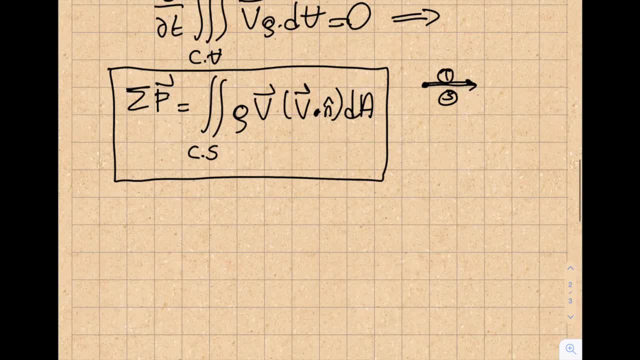 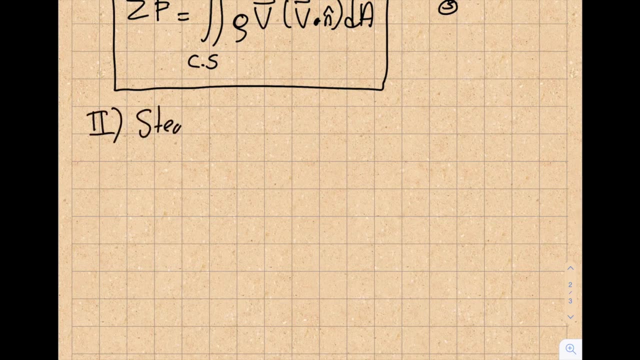 in here, but maximum, what I'm going to obtain if, in looking at this box of equation, is, if the density is out, it's going to be summation of the forces divided by density. it's not that special, okay. so then I'm gonna go ahead and make my second assumption as steady, and I'm 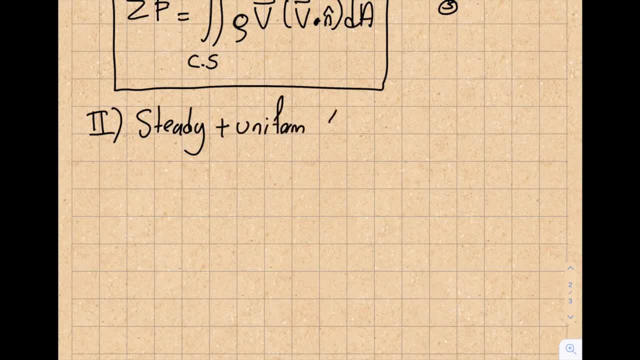 gonna add one more to it, which is called the uniform flow. okay, so also, I see some confusion for the definition of uniform flow, so let's discuss that for a minute here. uniform flow does not mean that the velocity is constant. okay, the uniform flow means that I have- let's. 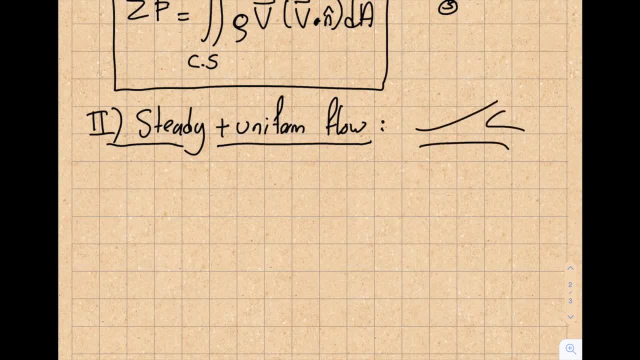 say that I have this shape right in an example: one inlet, two outlets. okay, and remember, vectors are defined at a point, not at an area. ok, when I say velocity at the inlet is equal to five meter per second, then I need to be much more specific and say: at the inlet, at this particular point, the 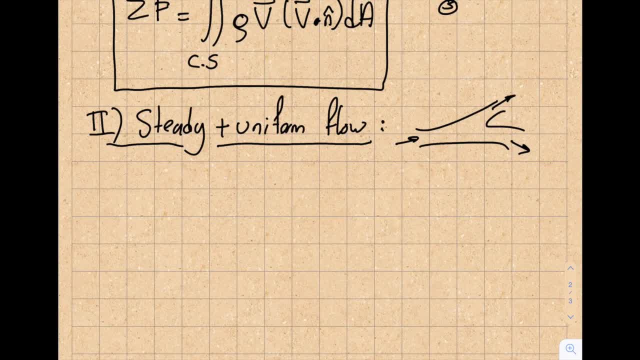 velocity is five. this uniform flow assumption will enable me to say that, hey, the velocity at the inlet, regardless of which particular point that I take, is the same. it doesn't change. ok. however, it doesn't say that this velocity will be equal to this velocity, all right. so now, if I go at the end with this steady and 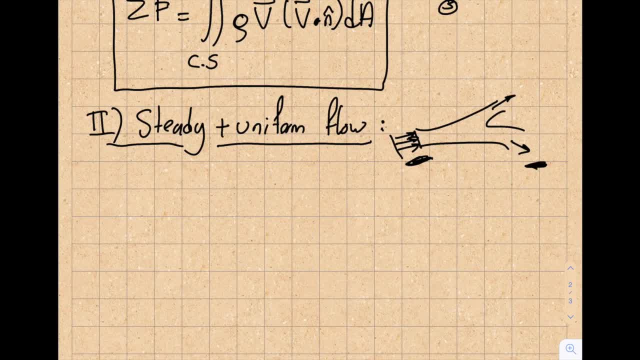 uniform flow assumption. what I'm going to have is the equation will. it will be the summation over the exits, what it will enable me to do. you can look at the video from the conservation of mass, how I obtained summation sign, because integrals, as you know, by definition are. we take small areas and we 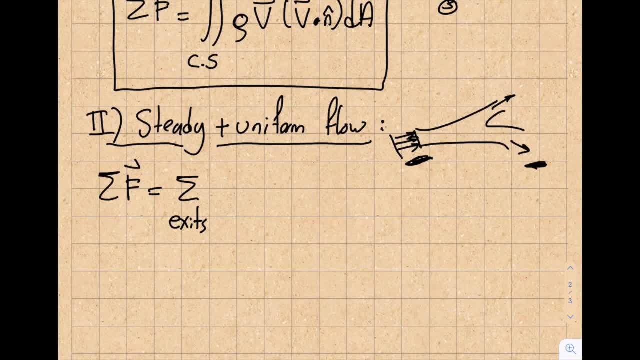 add them up. so I'm kind of going back to the definition of the integral ok row: exit V exit. Vn exit, a exit. ok, and I'll talk about this Vn exit in a moment. summation over the inlets row: inlet V inlet- Vn inlet a inlet- ok, now. 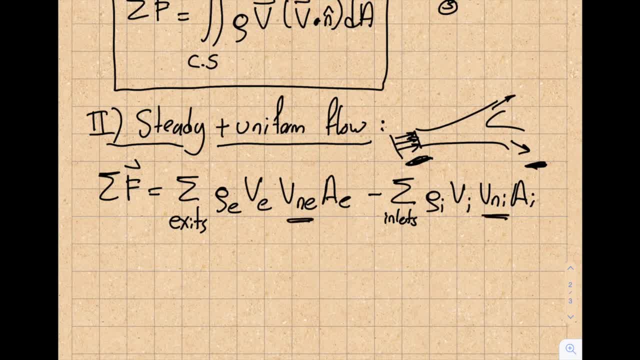 let's look at this n terms. this what what I mean by Vn is. I'm going to underline here as well, up there in the box of question. that's what what I mean by Vn. so this is the velocity at the inlet. ok, the velocity at the inlet and velocity. 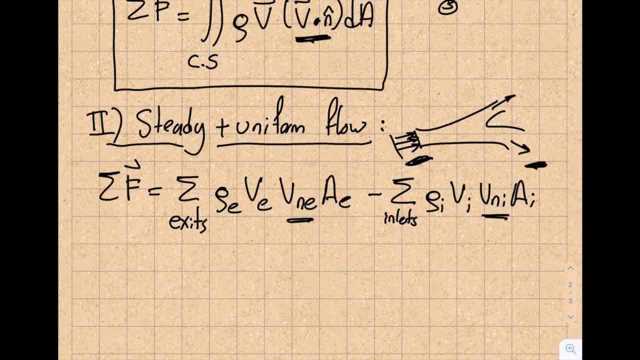 at the exit. but it doesn't have any components in the XYZ. it's in the normal direction. ok, at the exits. if you think about it, let's say this exit. you can see that the normals. if I'm drawing the normals over here in the figure, you can. 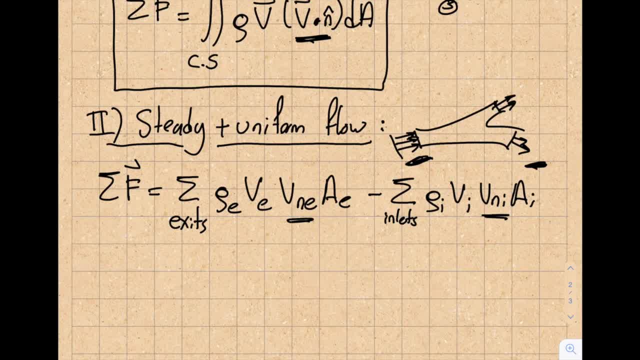 see that they are aligned with the velocity. so that's why I'm going to get a positive sign in front of the summation at the inlets. if you think about the normal, normal is pointing away from the surface right, but the velocity is to the into, so I'm going to get a negative sign. 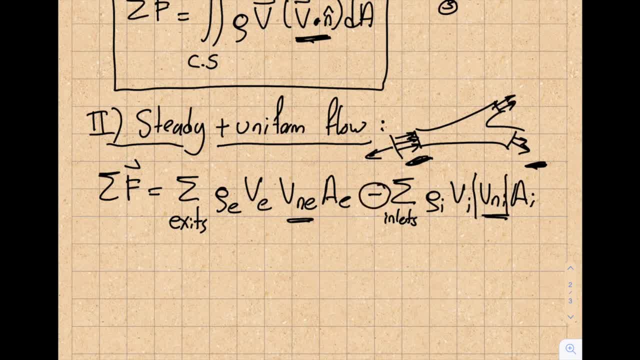 that's why this negative is, and so I would like you to be careful, and, although this is not an official way of representing this, I like you to think that there is no negative sign associated with either Vn inlet or Vn exit. granted, I do know that inlet is a negative. that's why I have the circled. 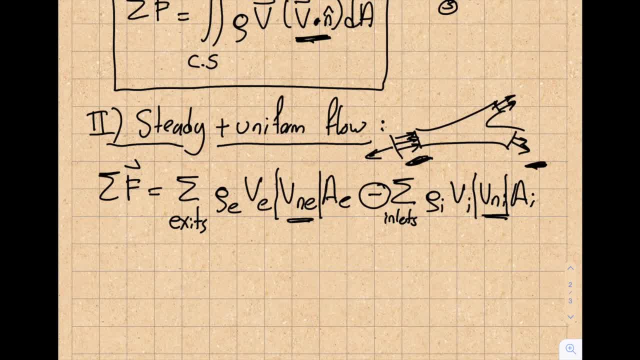 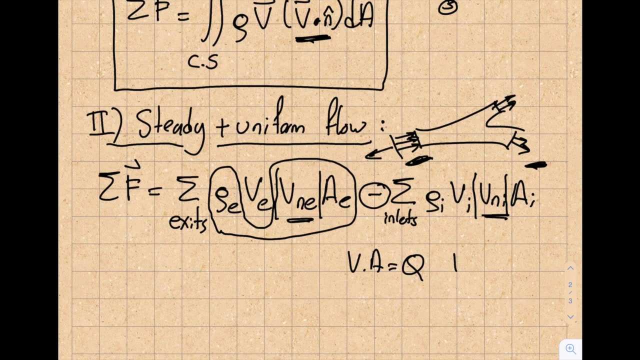 up negative sign over there. ok, so now we talked about this as well. so I'm going to actually like take these three terms and see what these multiplication of these three terms are: Rho, Va. ok, the multiplication of V times A. if you remember, V times A was the volumetric flow rate and, if I have V. 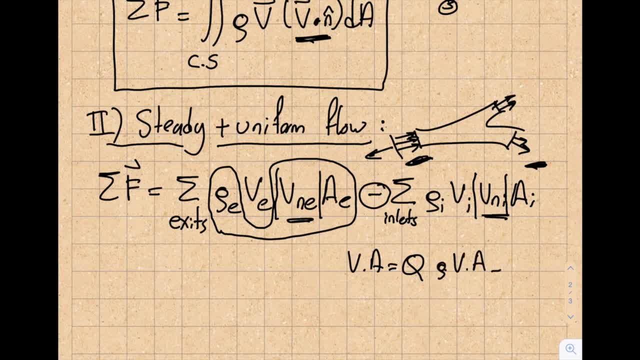 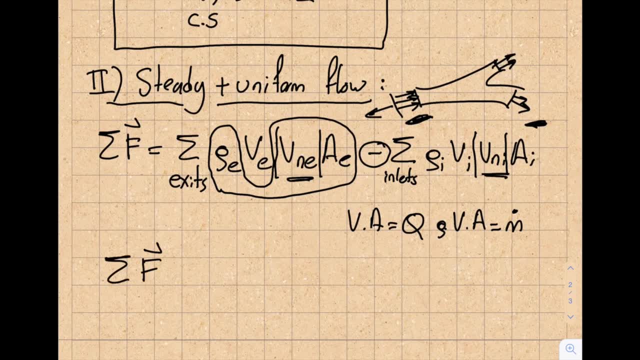 times A times density, that will be giving me the mass flow rate. ok, so I can simplify this equation further. it's not even simplifications, just for mathematical purposes. I'm going to have my exits as n dot, exit V, exit minus over the inlets and that inlet VI. okay, so this is another version. 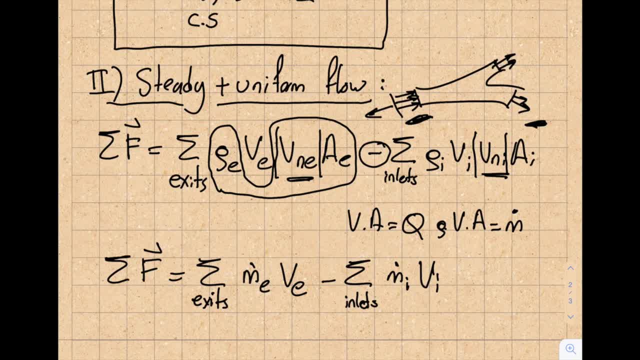 of this particular formula as well. the last thing I want to talk about is the left hand side of the equation. I didn't really need to talk about the left hand side of the equation. any of these assumptions, not particular to the assumption number two, a special case, number two, but any, any cases, I have to 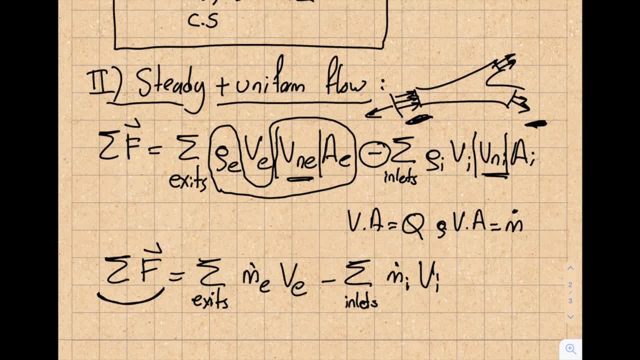 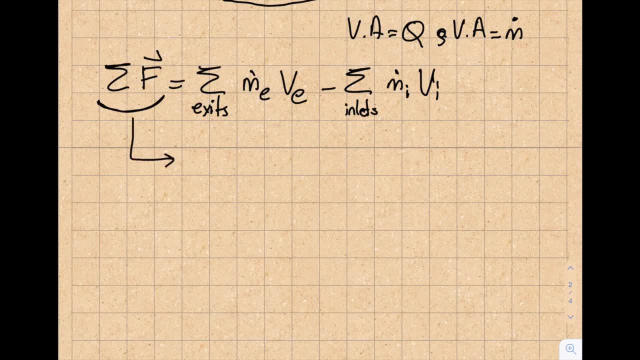 look at the forces, okay, and from our experience, what we noticed is there are three common types of forces that we have to account for in all of the cases, or we have an assumption for stating that this, this type of force doesn't exist. okay, and those three types of forces are first one. it's going to be. 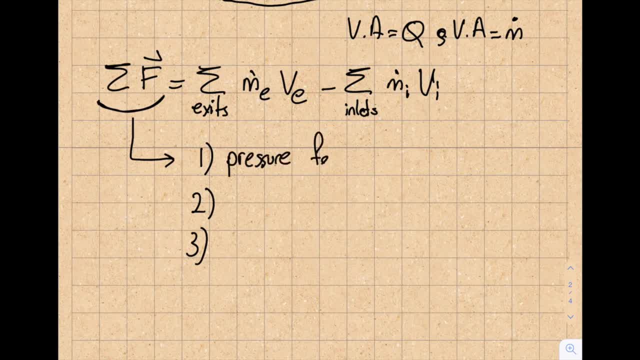 the surface forces and typical one is the pressure force. okay, if you think about the pressure force is P times a, so I need to know my pressure value. if I multiply by two, I get the pressure value. and if I multiply by two, I get the pressure value. and if I multiply by area, I'm gonna get a force. so I have to. 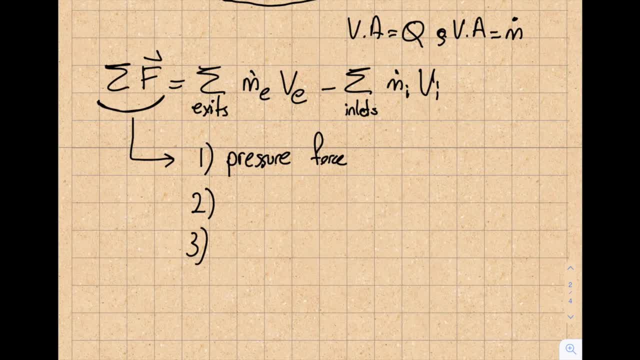 account for it. okay, and I want to talk about in here because I see issues say here as well. so let me write this particular example again, or rather draw again. I have an inlet here, I have an exit here and I have a exit over here. okay, as we discussed in the fluid static section as well, pressure always pushes. 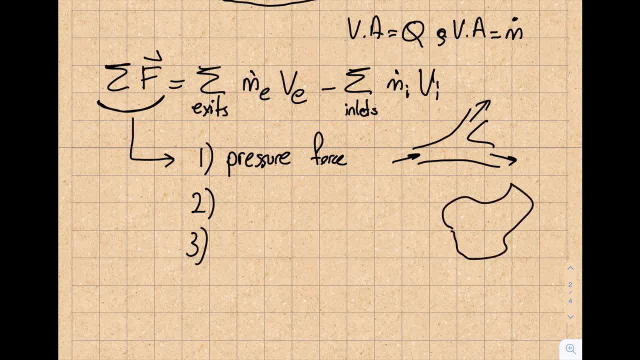 it in. if I have a balloon like this, any any particular shape, it always is perpendicular to the surface and pushes it in. so when I pick my control wall volume in a traditional way like that, what will happen is I have to indicate the direction of the pressures to be pushing into the surface. so if I draw 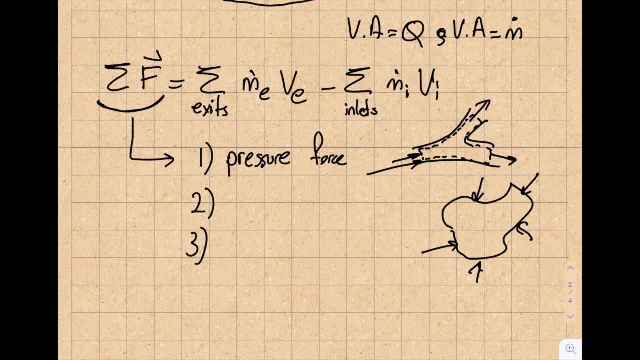 with longer arrows, so this is gonna be the P one a one. if, assuming this is section one, and careful, this is P 2 a 2, pointing it in, and this is P 3 a 3, pointing in as well. assuming this is section number three, this is section. 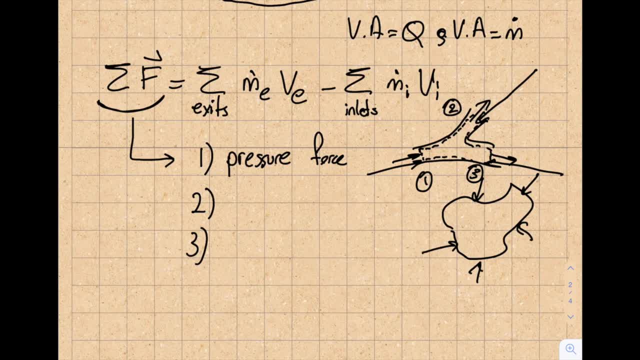 number two, and this is section number one. if I change the direction of the, the flow, let's say that two and three becomes an inlet and three becomes an exit. what happens to the direction of the pressure forces nothing, it still stays the same. note that the direction of 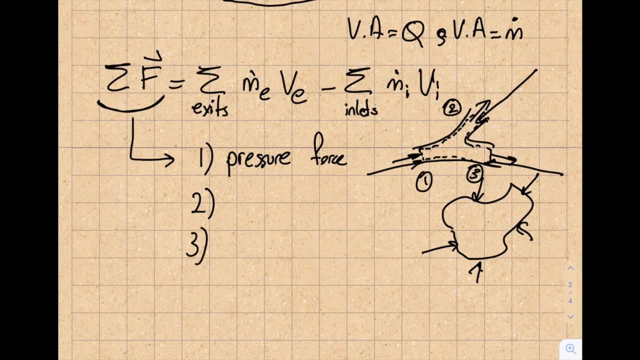 the pressure forces is nothing to do with the direction of the flow. i see these issues often from the students that didn't quite understand the topic. well, okay. the second force are viscous forces. okay, viscous forces are similar to friction in your salt mechanics courses. okay, when i have a. 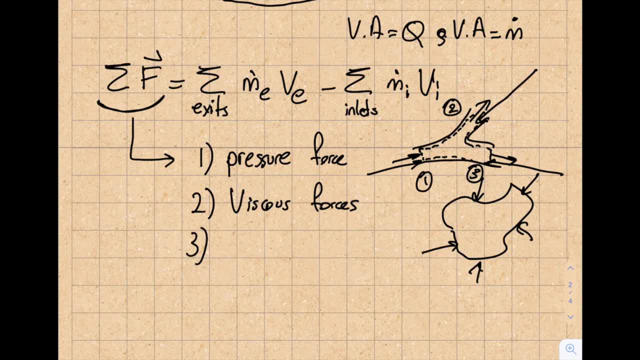 pipe. the flow is flowing in it. there will be some kind of a drag on it, right, it's gonna slow down. if i don't have a pump, you just turn off the pump, what will happen is the flow is gonna stop, right. that is the force stopping the flow in my pipe. okay, it's called the viscous forces and we touched. 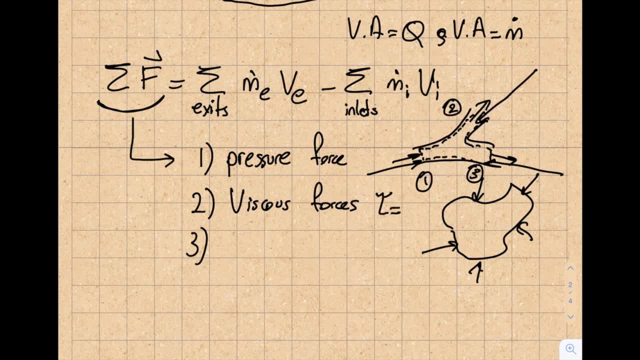 upon this in the first introductory concepts videos. so it's gonna be the viscosity times. du dy remember that, and if i multiply this by area, i'm gonna get myself viscous force that i should be incorporating to my analysis, and this viscous ίναι will be opposite to the direction of the flow. so now this one has something to do. 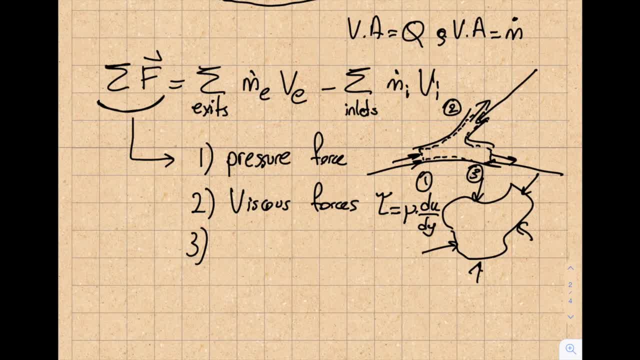 with the direction of the flow. okay, if you want to get rid of this particular force because you weren't given enough information, then I can just simply say this is inviscid flow. okay, and this is flow means that this is zero, so then I don't have to worry about viscous forces, okay. and the third one is: I want to call. 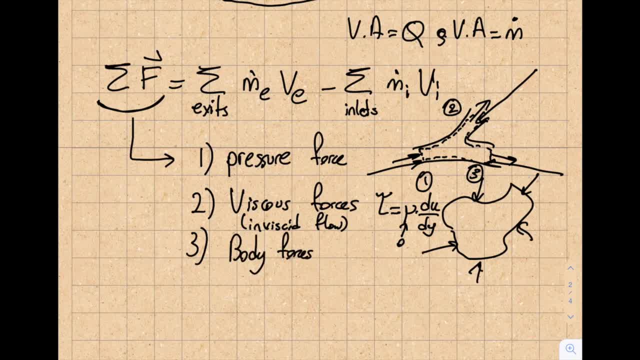 it body forces, but the most common one that we know of is the weight of the control volume. okay, the weight of the control volume. there's also magnetic forces. sometimes that acts on my flow. that's a body force, but that's not as common as the weight.